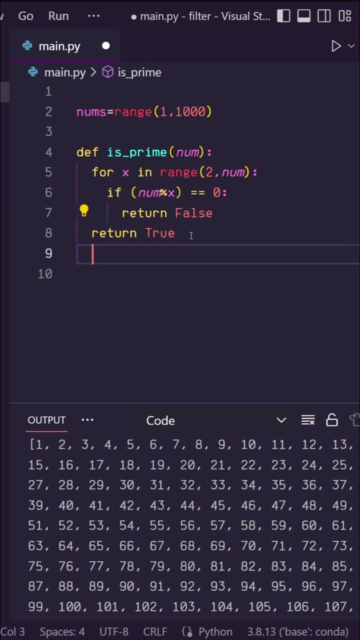 returns false if the number is not prime and returns true if it is. And now all I have to do is use Python's built-in filter function. I'll add isPrime and our list of numbers as inputs. Essentially, what this does is applies the isPrimes function to every item in the nums list. 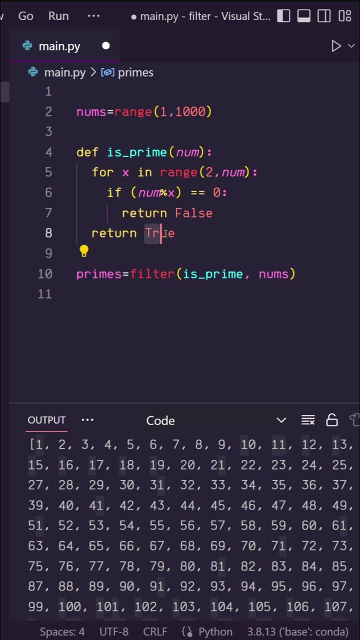 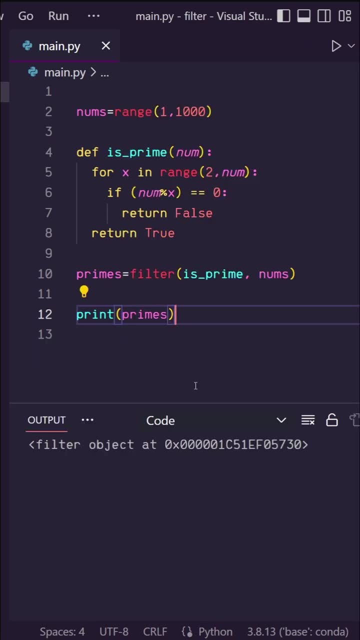 If a boolean true is returned, it stores it in our prime's variable. Otherwise, it removes the number And all we have to do now is print our prime's variable. However, you will see, it prints out a filter object. This is Python's way of conserving memory. 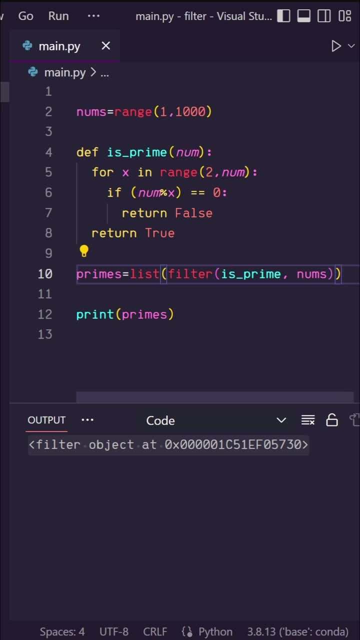 And so all I have to do is convert this to a list by putting this inside of the list function, And now we can run this, and there we go. We have every prime number from 1 to 1000.. Be sure to drop a like if you found this helpful. 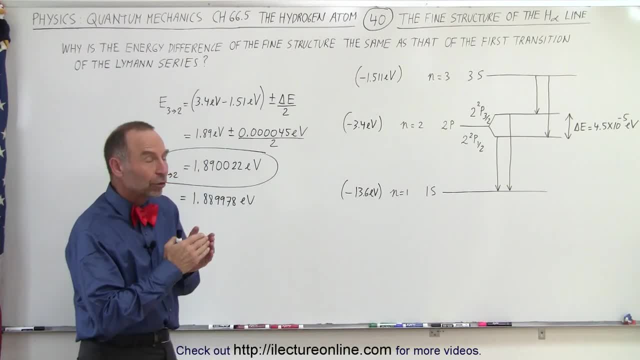 Welcome to Electron Line. In this video we're going to see why the H-alpha line energy difference in the fine structure is exactly the same as the first energy jump in the Lyman series, The first energy jump in the Lyman series from the second energy level down to the first energy. 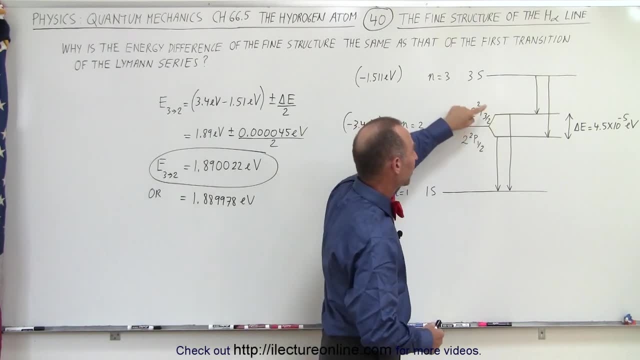 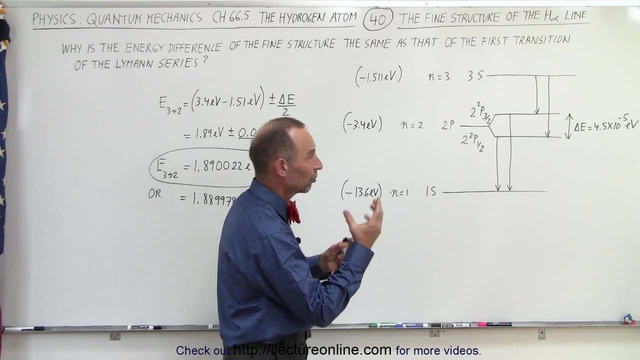 level in the hydrogen atom experiences energy difference because the fine line structure of the 2p orbital. In the 2p orbitals, when the electron orbits the nucleus, there's going to be a magnetic field created and then the interaction between the spin direction and the magnetic field. 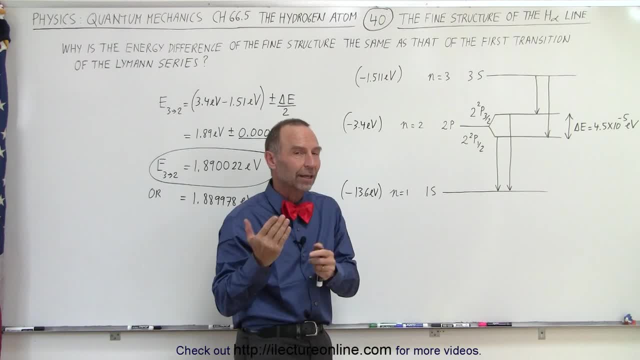 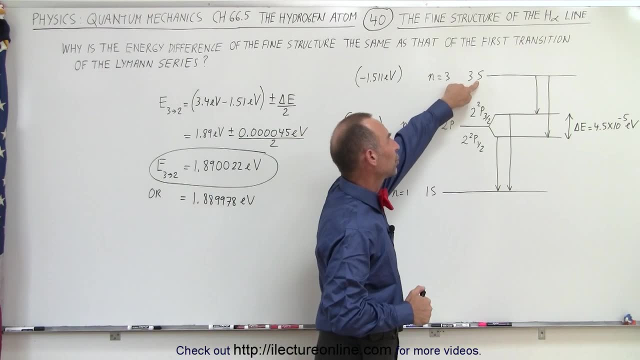 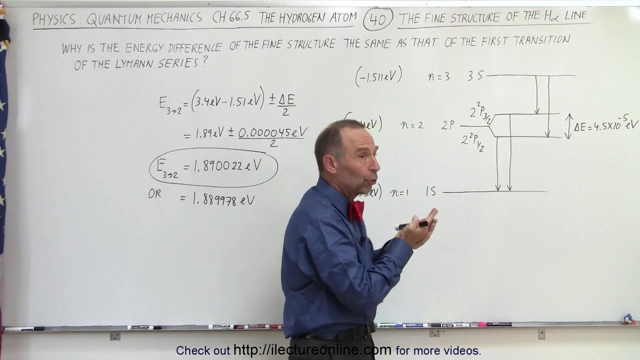 causes that slight difference in the energy, depending upon whether or not the electron is spin up or spin down. Well, when it jumps from the third energy level, it typically comes from the 3s orbital, and there you do not see that fine structure difference because it's an s orbital. 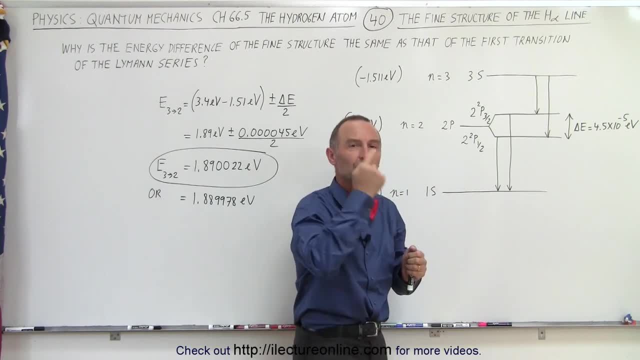 and in an s orbital there's an equal probability that the electron will travel around the nucleus in any given direction And because of that there's no magnetic field created and therefore we don't have that interaction between the spin direction of the electron and the non-existing magnetic field.